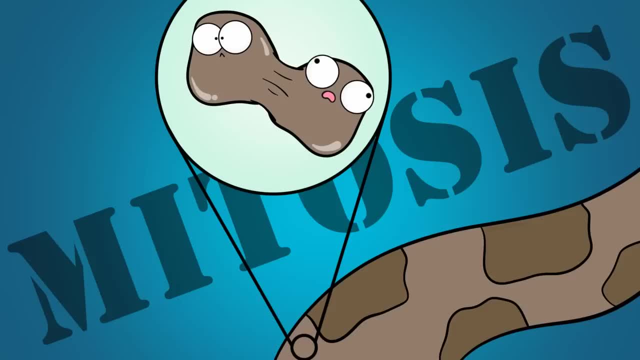 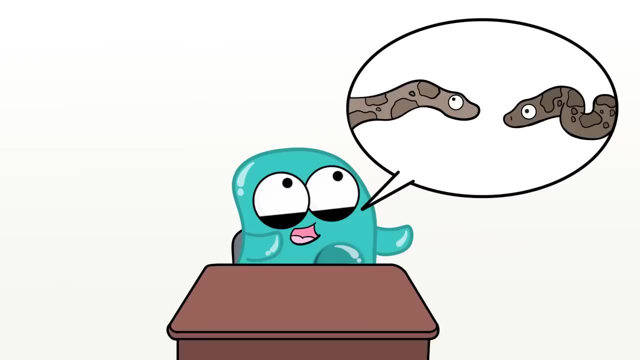 Mitosis. Let's talk about why Spike even needs to make more cells. One day in tutorials I said: I'm going to teach you how to make more cells. A student asked me: since Spike's parents were bred in captivity, did you ever see Spike's parents? Do you think Spike's parents looked like him? 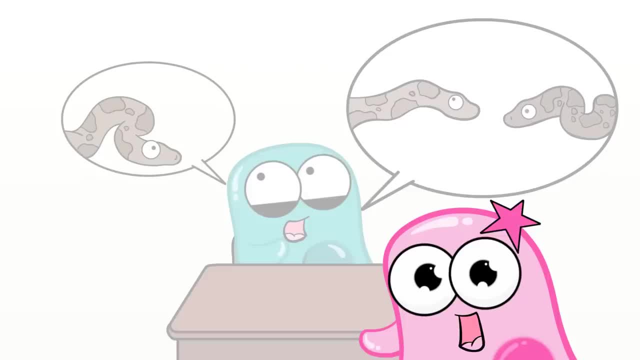 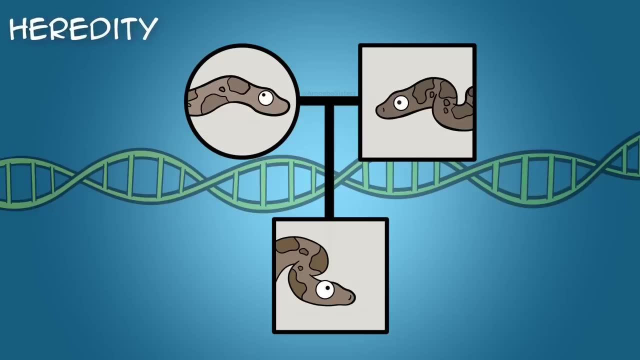 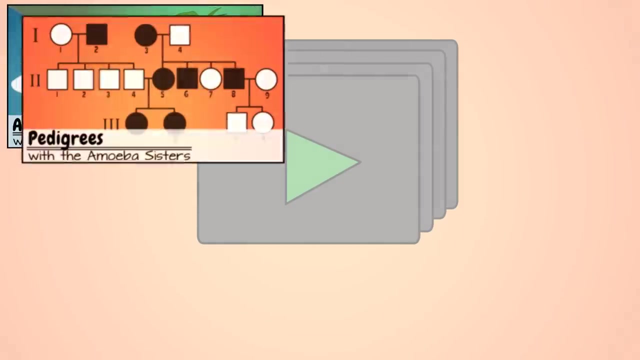 You can't ask a question like that and not expect an answer. It was a great question because we were getting close to our heredity unit. Heredity is about how traits are passed down from parent to offspring. We've made a playlist of our videos that focus on heredity, including reproduction, how to track inheritance and pedigrees, how to solve genetic problems in Punnett Squares. 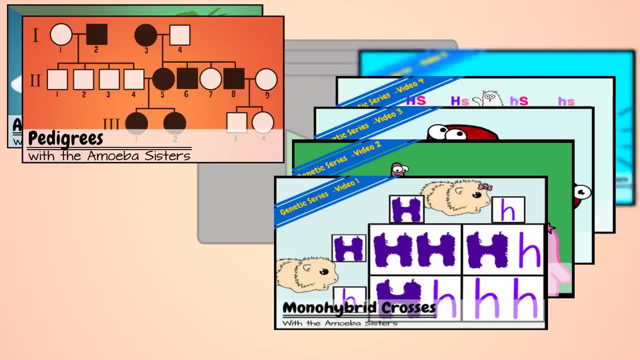 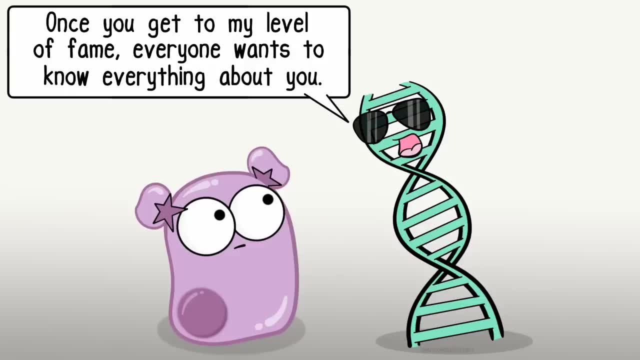 and how to make a family And understanding different Mendelian and non-Mendelian inheritance. But you really can't delve into those and study heredity without understanding DNA, chromosomes, genes and traits, And that's what this introductory video is going to focus on. 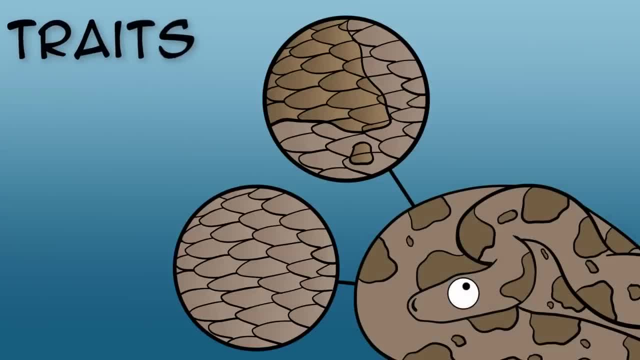 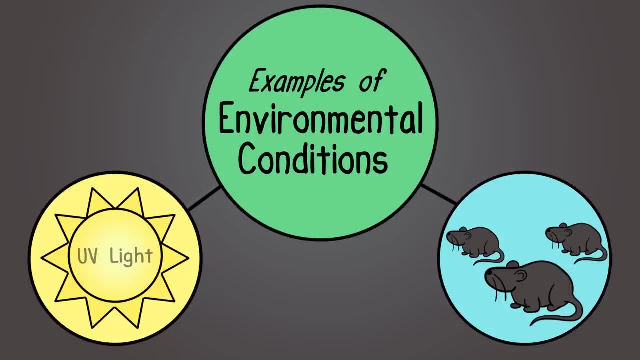 So back to the student question. Spike has traits, The patterns on his body, his size. these traits are coded for in his DNA. Some of the traits he inherited can be influenced by the environment. For example, if Spike had not had the nourishment he needed, that could affect his size. 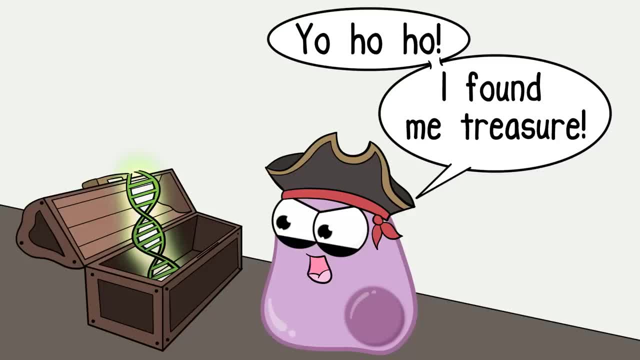 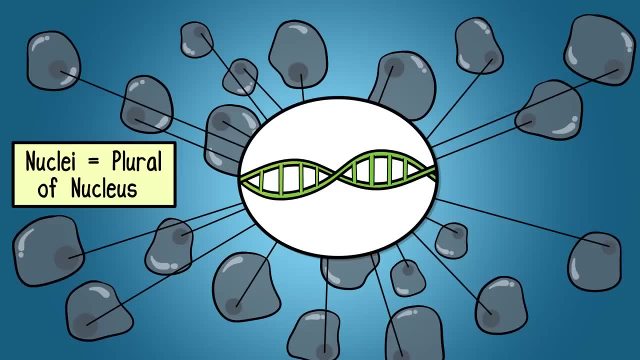 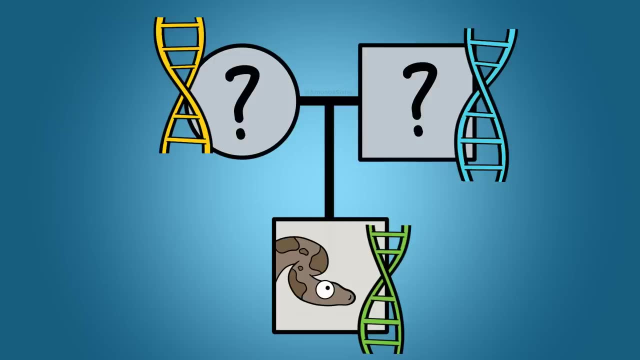 DNA is not just one big code buried deep down in an organism like some treasure. Spike's DNA is in the nuclei of nearly all of his body cells. He inherited his DNA from his mother and father. I can't know for sure what Spike's parents looked like, but I do know that Spike inherited his DNA from them. 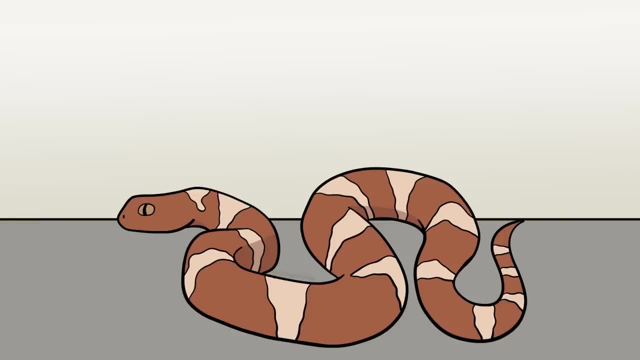 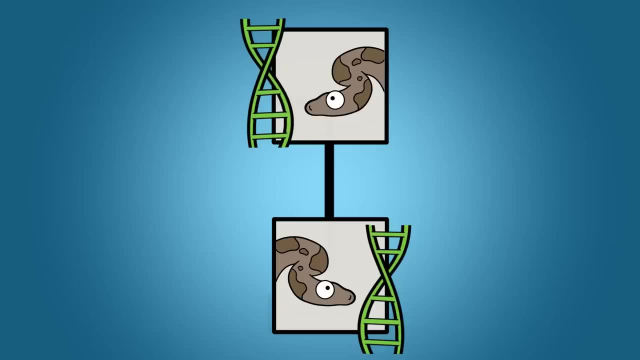 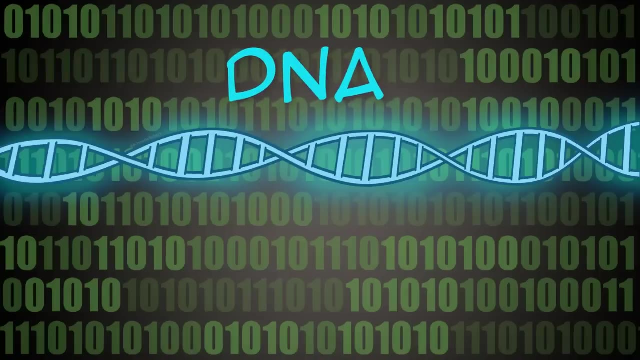 One fun fact: many snake species can reproduce asexually. Had that been the case for Spike, he would have inherited all of his DNA from only one parent, But it would still be DNA coding for traits. Just like Spike, your DNA codes for your traits. 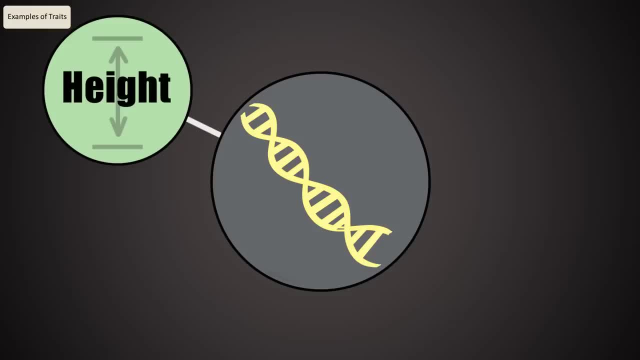 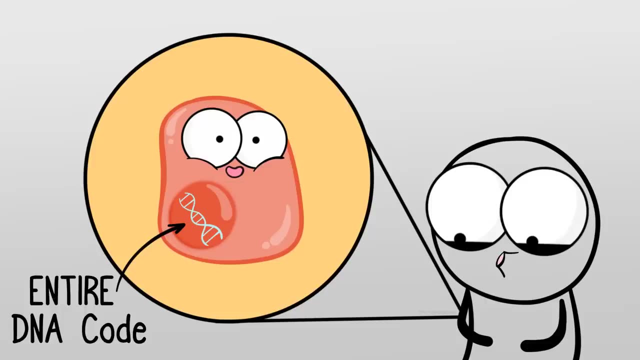 And your cells can't function without it. DNA determines how tall you are, what color your eyes are, what color your hair is, or even if you're at risk for certain diseases Also like Spike, your entire DNA code is in most of your body's cells. 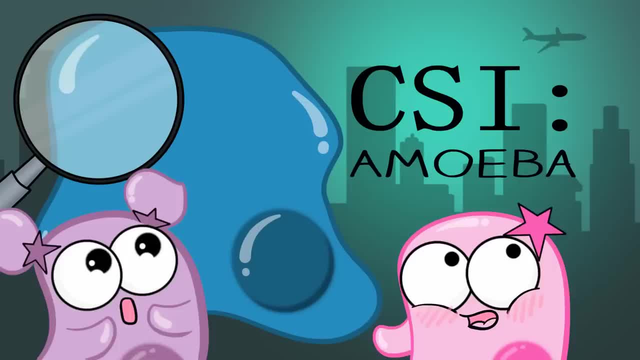 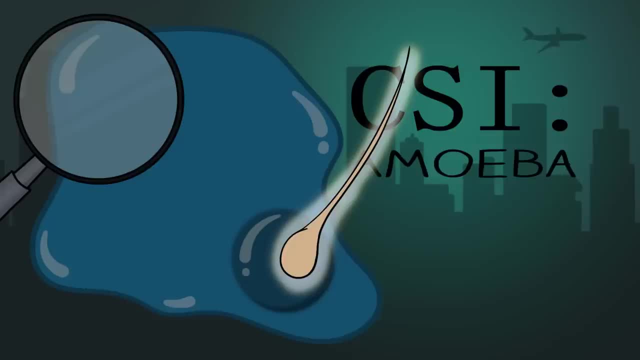 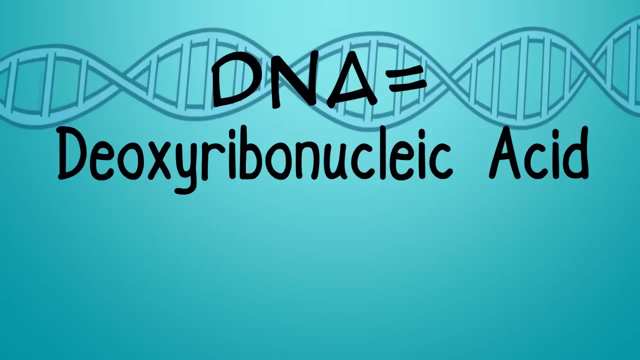 That's why, in crime-solving shows which we may or may not absolutely love, a criminal can sometimes be caught by just leaving a cell from a hair follicle behind DNA has a beautiful structure, And that structure will help you understand how inheritance works. 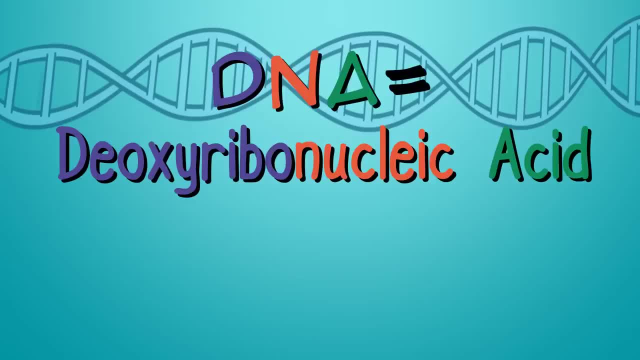 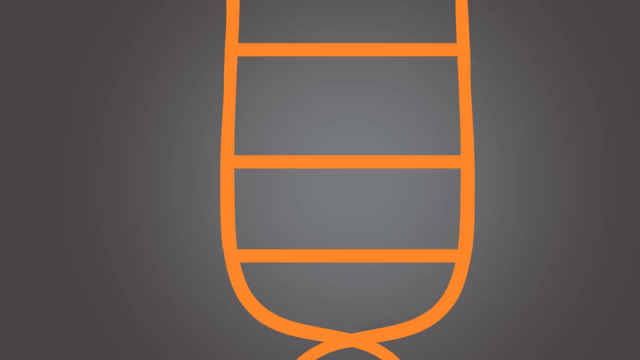 DNA stands for deoxyribonucleic acid. It's a type of nucleic acid. If you remember from our biomolecules video, nucleic acids are a type of biomolecule. Nucleic acids are made up of building blocks called nucleotides. 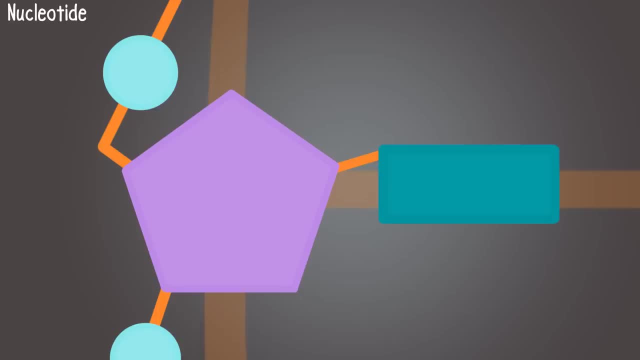 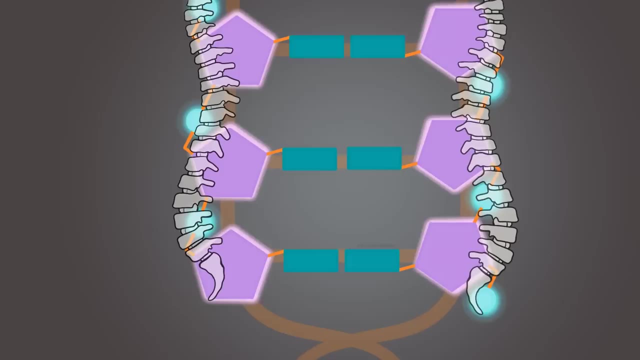 Nucleotides have three parts. One of them is a sugar called deoxyribose. One of them is a phosphate. We sometimes say DNA has a sugar-phosphate backbone, But the most important part of the nucleotide is the base. 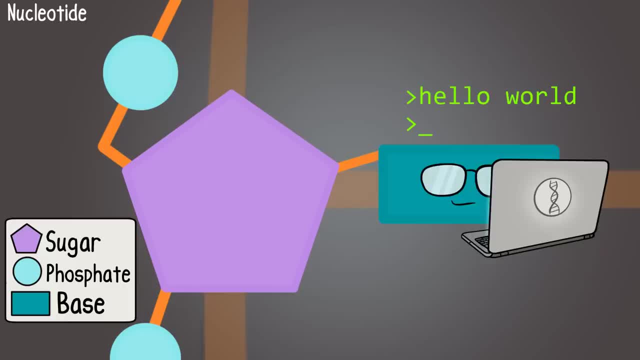 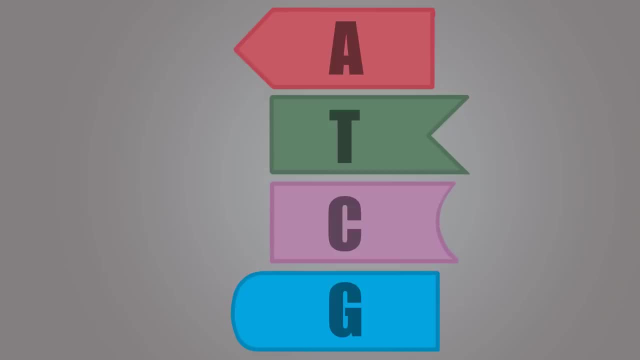 Because the sequence of the bases can actually code for traits. So, as far as the bases go, there are four types of bases in DNA. A lot of times they'll just use the letters A, T, C, G. The A is for adenine. 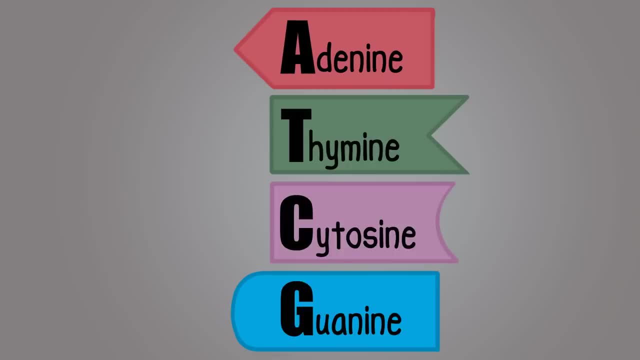 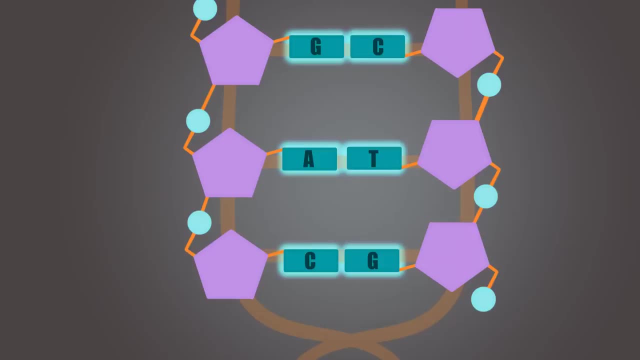 The T is for thymine, The C is for cytosine And the G is for guanine. These bases actually pair in a specific way, And there's a popular mnemonic that can help you remember which of them pair together. Apples in the tree. 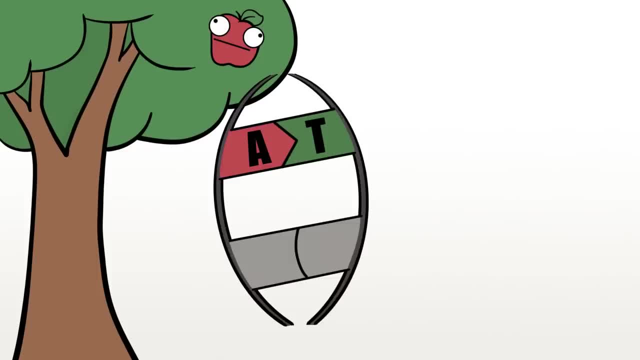 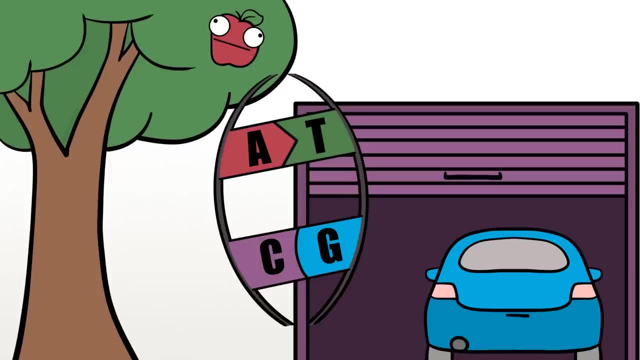 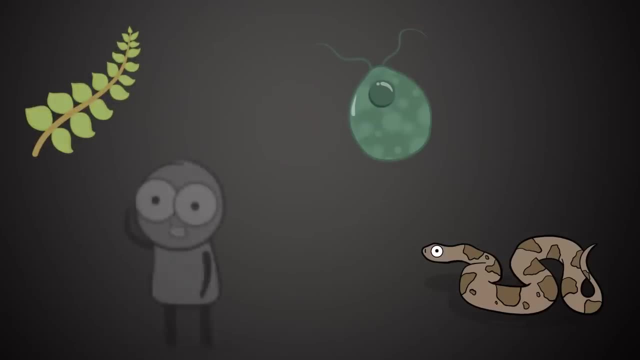 That tells you the A for apples, T for tree, Because the bases A and T go together. The other verse is car in the garage And that can help you remember: the base C always goes with the base G. So whether we're talking about Spike or a plant, or a protist or a human like you, 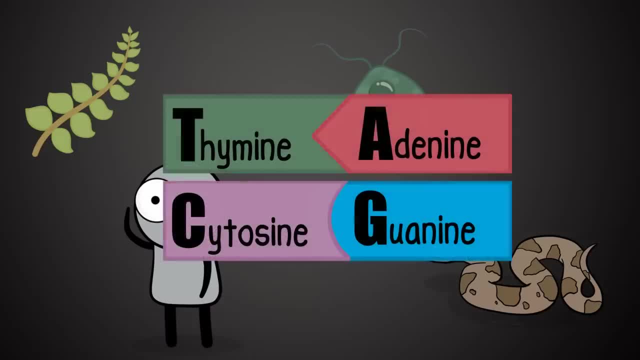 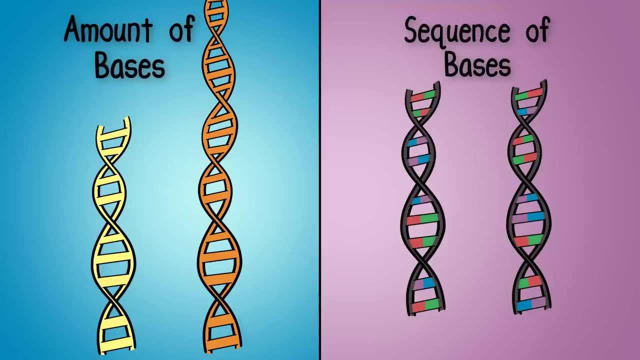 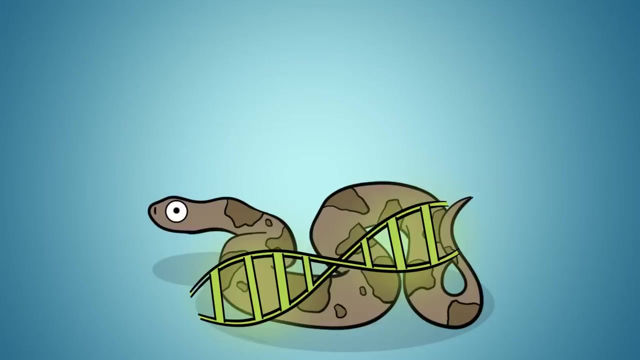 these are the DNA bases in living organisms, But the amount of DNA bases overall and the sequence of those bases we mentioned will vary among different species And also among different individuals, But it's likely to infer that Spike has a sequence of DNA bases that is more similar to his parents. 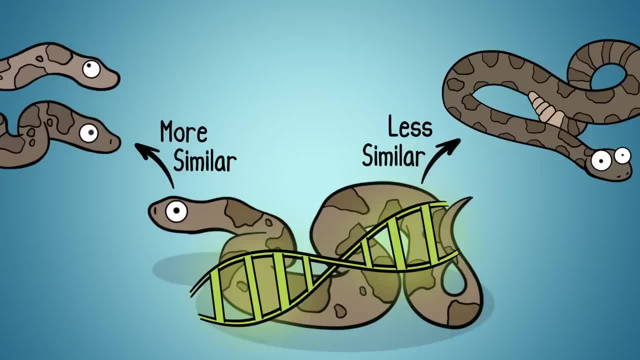 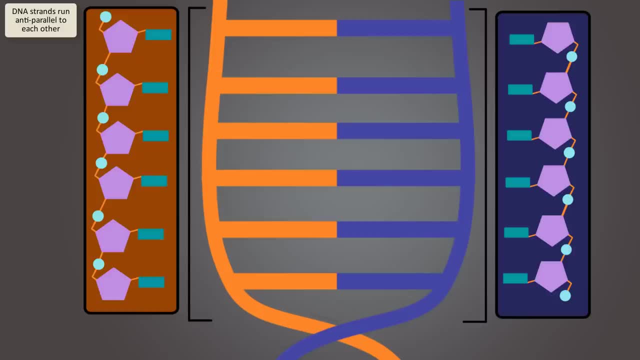 than he would to say a rattlesnake. DNA has two strands, So there are nucleotides running up one side and there's nucleotides running up the other side. The bases are what pair in the middle? The bases are held together by hydrogen bonds. 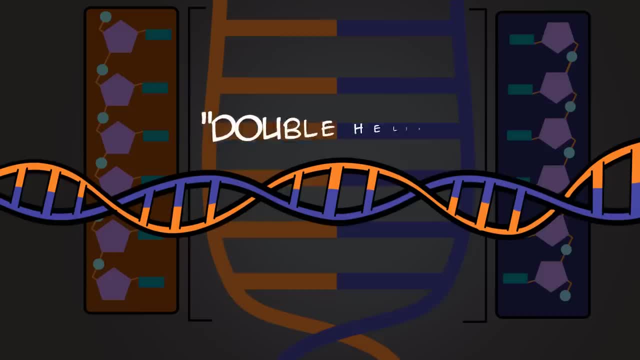 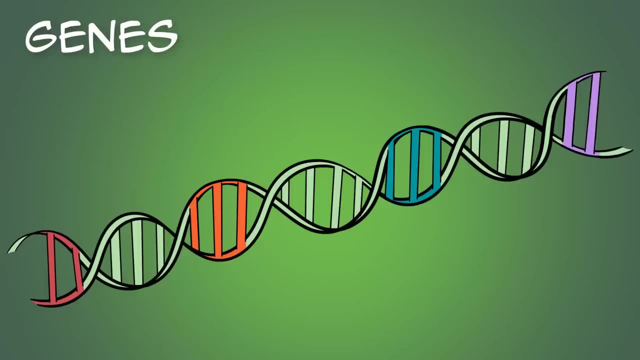 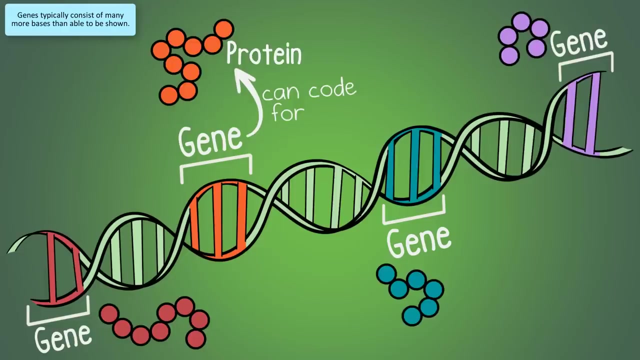 The DNA is also twisted in something we call a double helix shape. Portions of DNA make up genes. We can say, for example, that this part of the DNA here makes up a gene. Genes can code for proteins. Proteins have a huge role in expressing a trait. 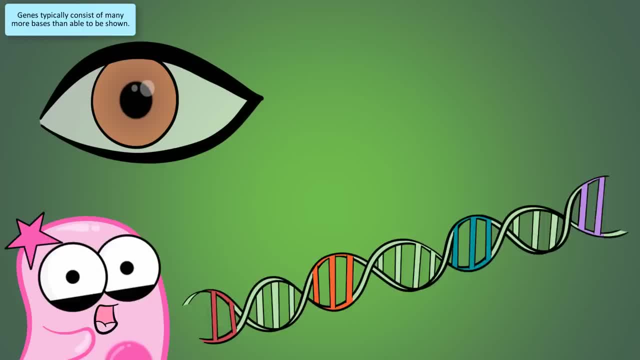 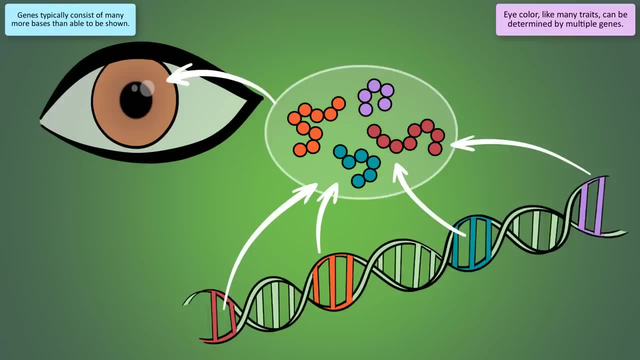 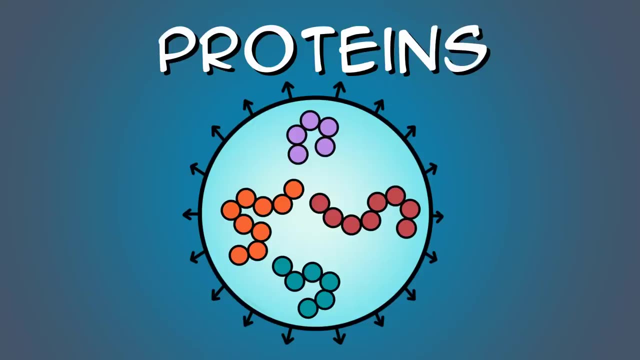 For example, let's consider your own eye color. Human eye color is actually pretty complex. It's determined by many genes. The genes can code for proteins involved in producing the eye color pigment. But proteins coded for by genes, They can play a wide variety of roles besides just your eye color. 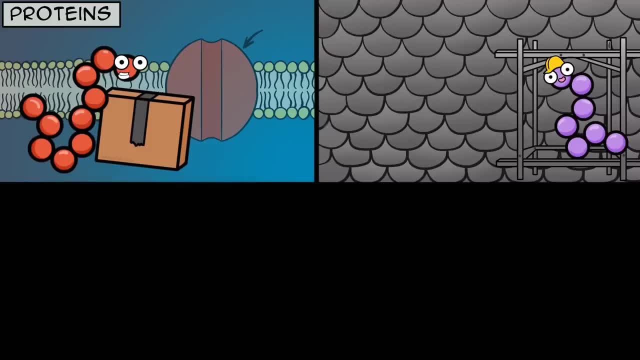 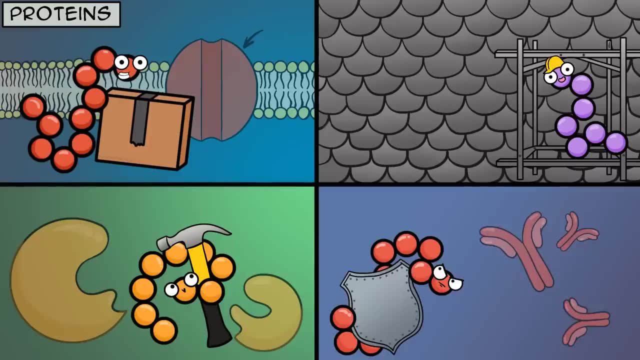 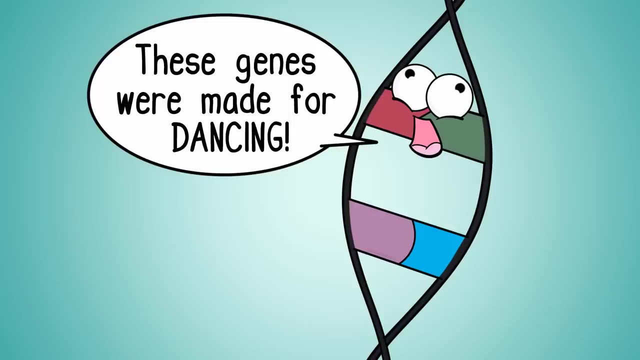 Proteins are involved in transport, in structure, in acting as enzymes that can make all kinds of materials, in protecting the body and so much more, And that not all genes are used to make protein And there are parts of DNA that are non-coding. 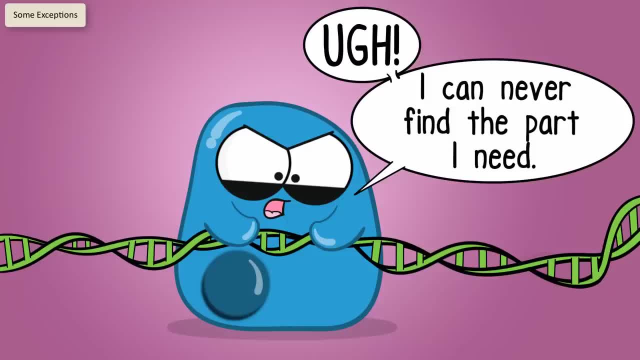 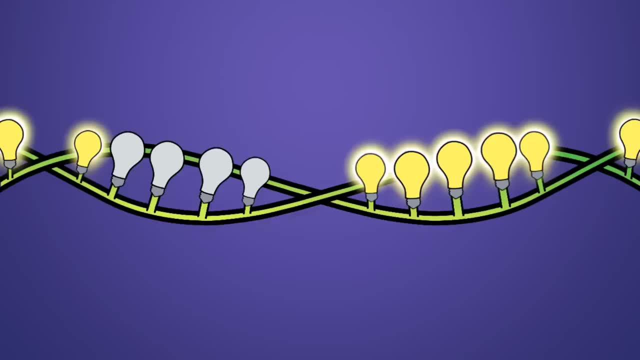 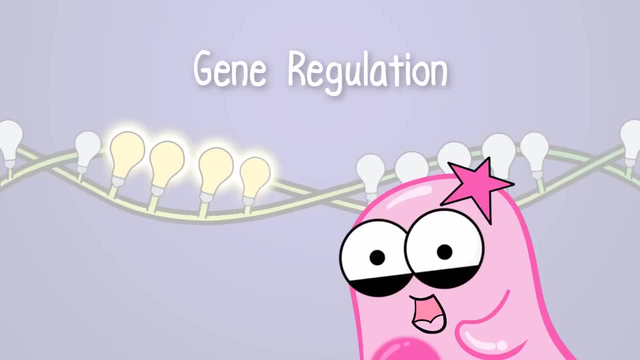 And even though nearly all of your body cells have your entire DNA code, your body cells may only use certain portions of those genes. Genes can be turned on or turned off by a variety of mechanisms. We call that gene regulation. Check out our video on that. 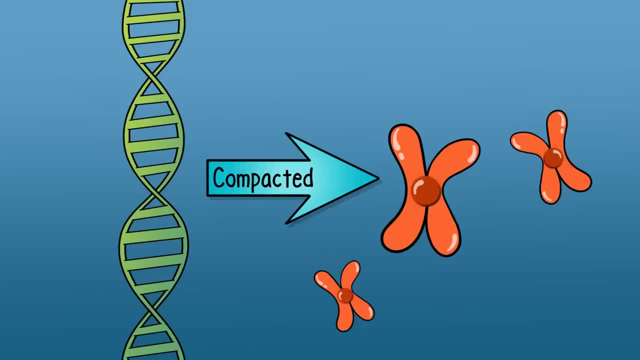 Now you have a lot of DNA. When it's compacted it's organized into a unit called a chromosome- Very helpful when you're trying to make more cells and you need to get the DNA into those new cells. Chromosomes in your body involve DNA wrapped around protein structures. 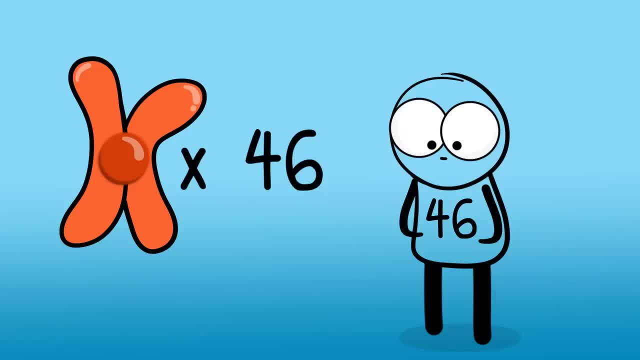 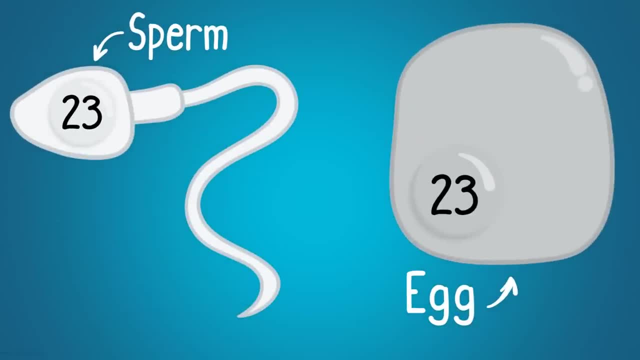 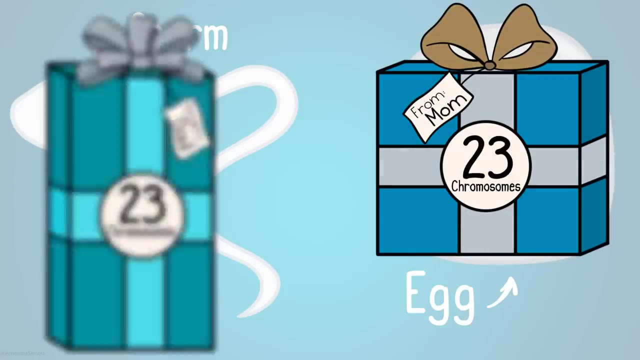 Humans have 46 chromosomes. That means nearly every body cell in your body has 46 chromosomes. Human sperm and egg cells, on the other hand, each contain 23 chromosomes. So you receive 23 chromosomes from your mother, 23 chromosomes from your father. 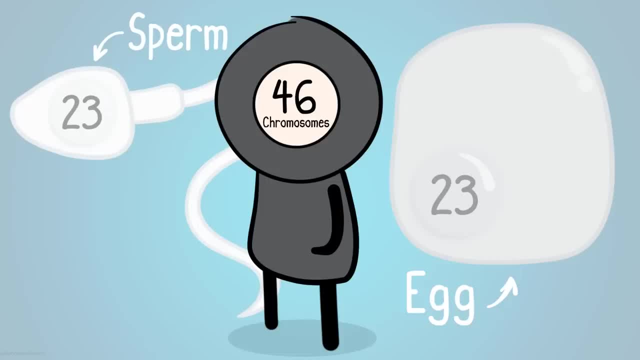 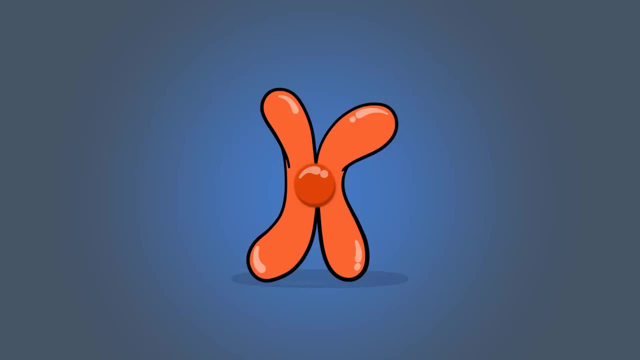 24 chromosomes from your father to give you your 46 chromosomes, Your genetic code. So let's do a recap of the big picture. Here's a single chromosome. You see genes on this chromosome. These genes consist of portions of DNA. 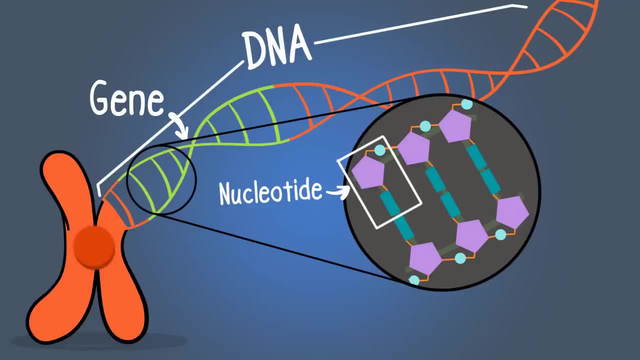 DNA is made up of nucleotides. DNA is made up of nucleotides And it's these bases here, the sequence of them, that makes the difference in coding for traits. that makes the difference in coding for traits Phew. 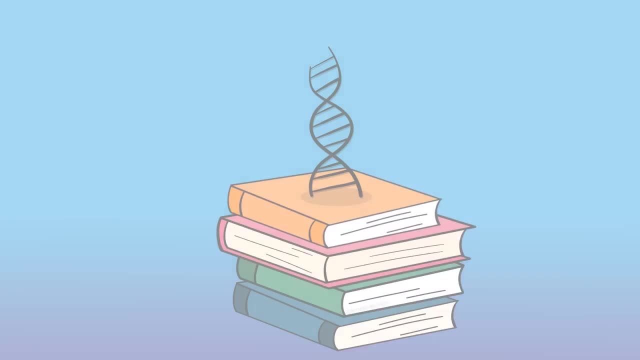 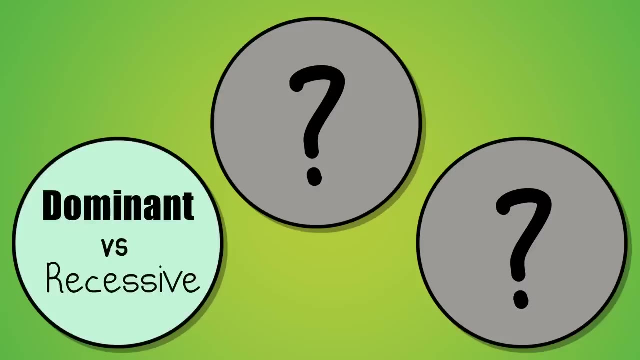 Understanding this foundation is essential in understanding heredity, whether you're talking about you or Spike. So this may bring up more questions now, like: where do dominant and recessive traits come in? like: where do dominant and recessive traits come in?